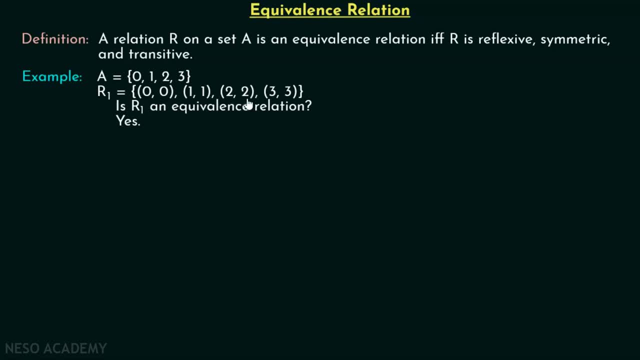 Then we have an ordered pair 1, 1.. Then we have an ordered pair 2, 2.. And finally we have an ordered pair 2, 2.. And finally we have an ordered pair 3, 3.. 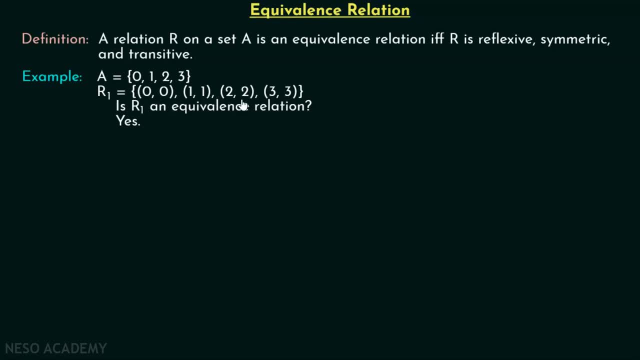 So this relation is reflexive, Then obviously this relation is symmetric and transitive. There is no doubt about this. You can check this on your own. Therefore, this relation R1 is an equivalence relation, because all these three properties are satisfied for this relation. 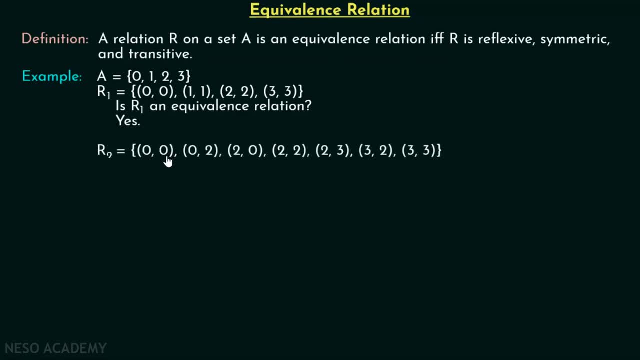 Right, Let's see R2, which consists of these ordered pairs: 0, 0, 0, 2, 2, 0, 2, 2, 2, 3, 3, 2, 3, 3.. 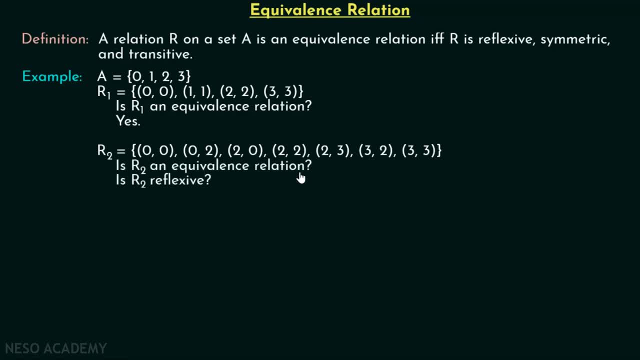 Is R2 an equivalence relation? First we must ask this question to ourselves: Is R2 reflexive? See this: We have this ordered pair 0, 0.. Fine, We have an ordered pair 2, 2.. Then we have this ordered pair 3, 3.. 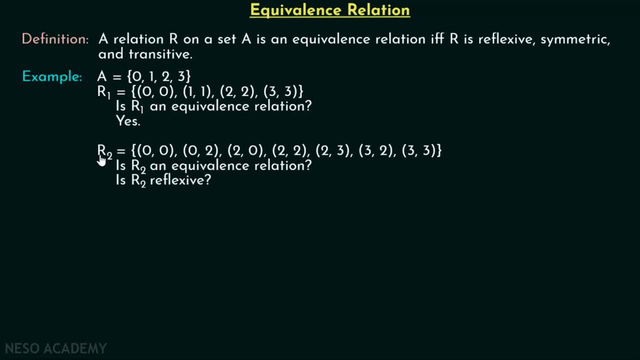 But there is no ordered pair 1, 1 in this relation Right. Therefore, this relation is not reflexive. Because 1, 1 is not a member of R2, therefore this relation is not reflexive. There is no need to check any other property. 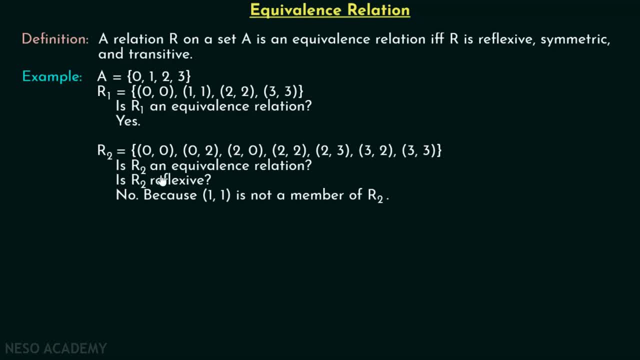 Right, This relation is not reflexive, So it is clear that this relation is not an equivalence relation. Fine, Now let's see R3, which consists of these ordered pairs: 0, 0, 1, 1, 2, 2, 1, 2, 2, 3, 3.. 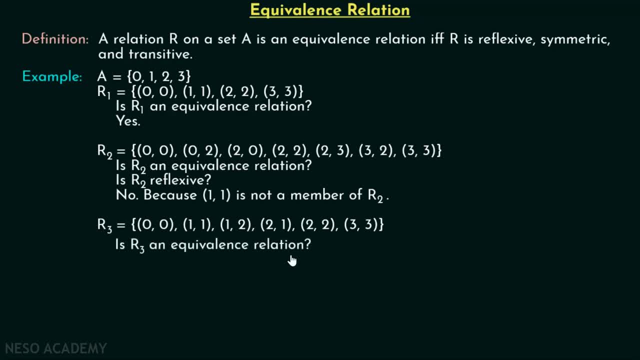 These are all the ordered pairs of this relation R3.. Is R3 an equivalence relation, Ask yourself. is R3 reflexive? You can see we have these ordered pairs: 0, 0,, 1,, 1,, 2,, 2, 3, 3.. 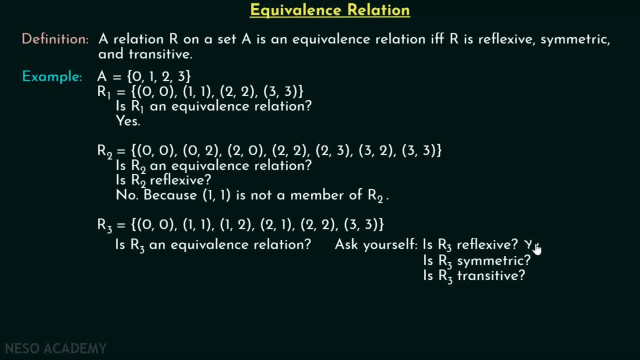 Obviously this relation is reflexive, Right. So R3 is reflexive. Now is R3 reflexive, Is R3 symmetric? You can see that for 1, 2, we have 2, 1. Right. 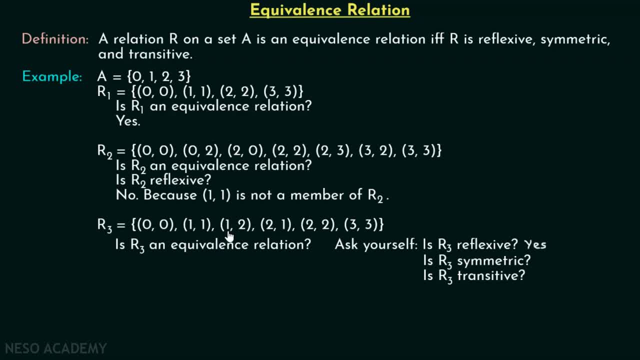 For the rest of the ordered pairs there is no need to check, But for this ordered pair that is 1, 2, there must be 2, 1 in this relation R3.. And you can see that 2, 1 is there. 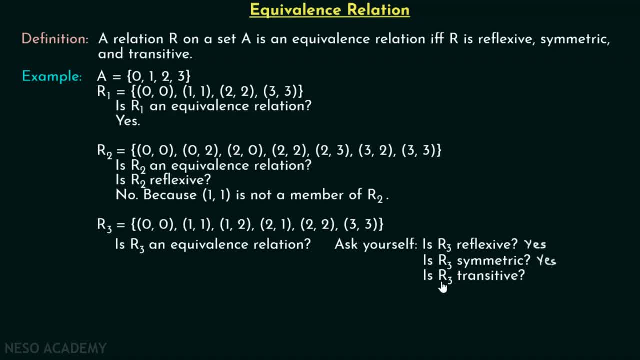 Therefore, this relation is symmetric. Right Is R3 transitive. For 1, 2 and 2, 1, we obviously have 1, 1.. For 2, 1, 1, 2, we have 2, 2 in this relation. 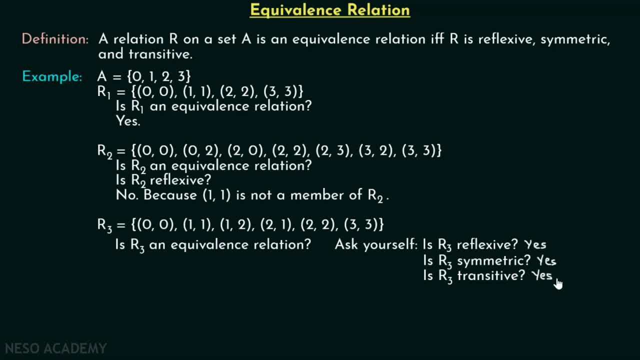 Obviously, this relation is transitive as well. Right, Therefore, R3 is an equivalence relation. This relation, R3 is reflexive, symmetric and transitive. therefore, relation R3 is an equivalence relation. Right Now let's see relation R4.. 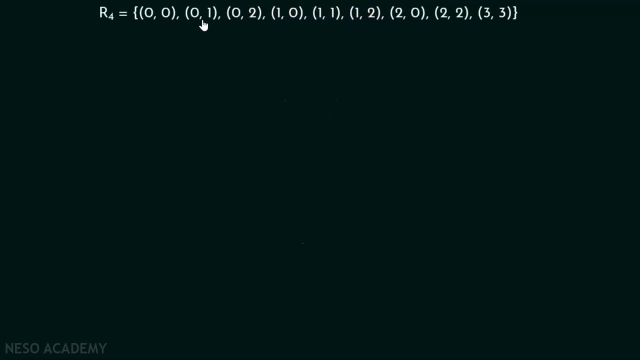 This is relation R4, which consists of these ordered pairs: 0, 0, 0, 1, 0, 2, 1, 0, 1, 1, 1, 2, 2, 0, 2, 2, 3, 3.. 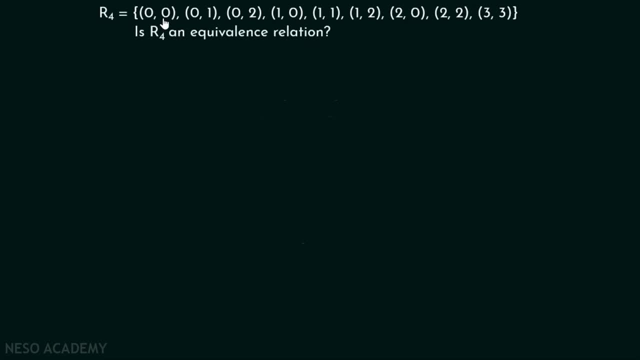 Is R4 an equivalence relation? Is this relation an equivalence relation, Ask yourself. is R4 reflexive? Yes, you can see: 0, 0 is there, 1, 1 is there, 2, 2 is there, 3, 3 is there. 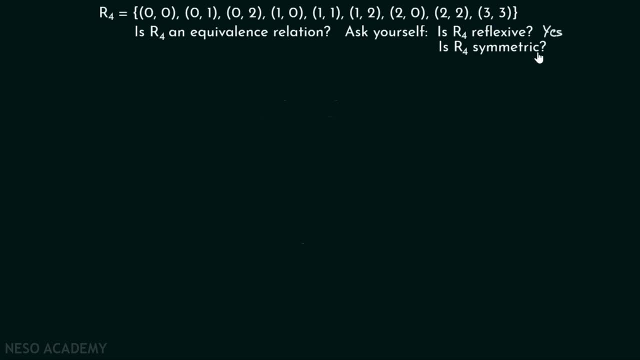 Obviously, this relation is reflexive. Right Is R4 symmetric. Okay, let's check this. We have 0, 1.. For 0, 1, 1, 0 must be there in this relation. You can see 1, 0 is there. 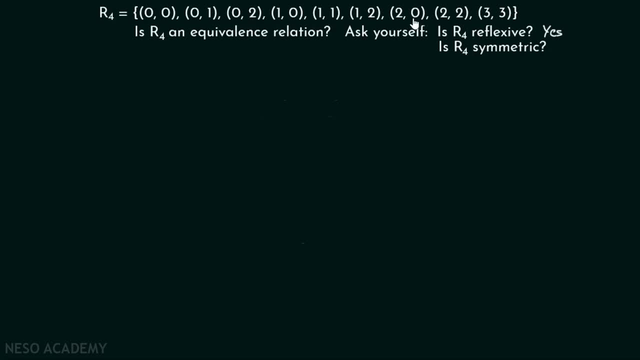 Okay For 0, 2,. 2, 0 must be there in this relation. You can see 2, 0, is there? Fine, For 1, 2,. we must have 2, 1 in this relation. 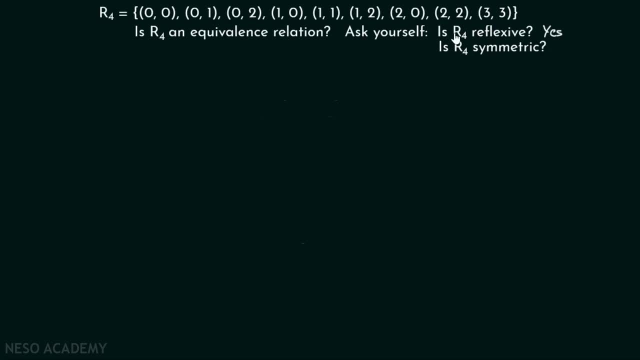 You can see that there is no ordered pair 2, 1 in this relation. Therefore, this relation is not symmetric, Fine. Hence it is clear that R4 is not an equivalence relation. Right Now let's see relation R5.. 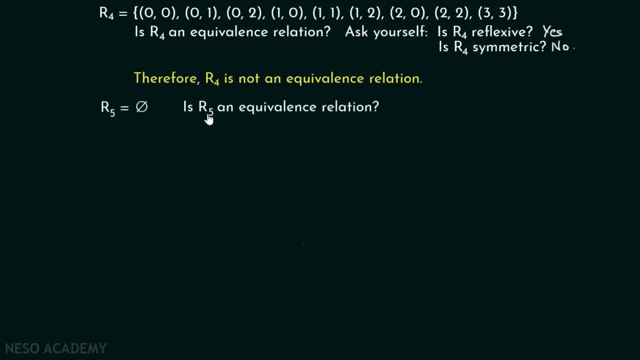 Here, R5 is nothing but an empty set. Is R5 an equivalence relation? Ask yourself: is R5 reflexive? No, Right, We know that R5 is not reflexive. An empty relation is not reflexive, Right. 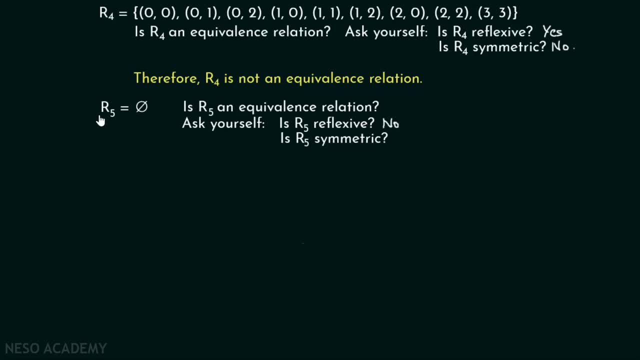 There is no need to check whether R5 is symmetric or not. We can clearly say that R5 is not reflexive. Therefore, R5 is not an equivalence relation. As simple as that. Right Now, let's see relation R6.. 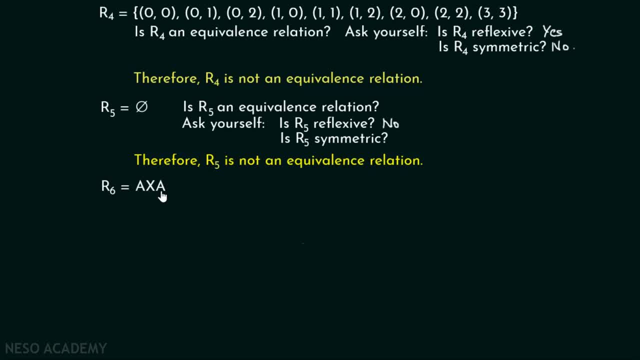 R6 is nothing but A cross A Fine. Is R6 an equivalence relation? Ask yourself, is R6 reflexive? Obviously, A cross A is the largest possible relation, Right. It must include every ordered pair, Right. Therefore, this relation must be reflexive, symmetric and transitive.